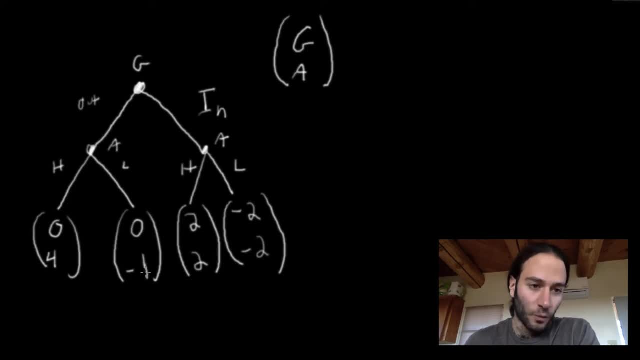 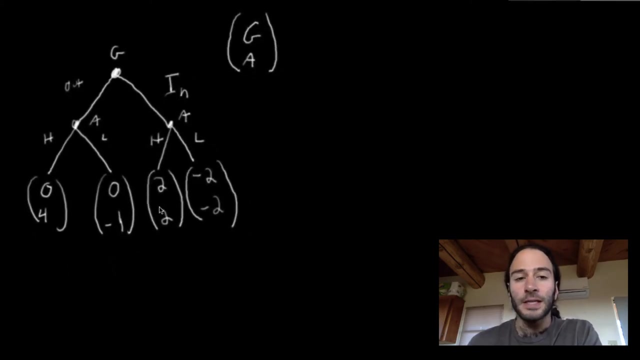 Apple plays out well. would Apple want four or negative one? Well, it would probably want four. You know, higher is always better. So in this case we see that, no matter what Google does, Apple would most likely choose the high price. Okay, Let's look at a certain 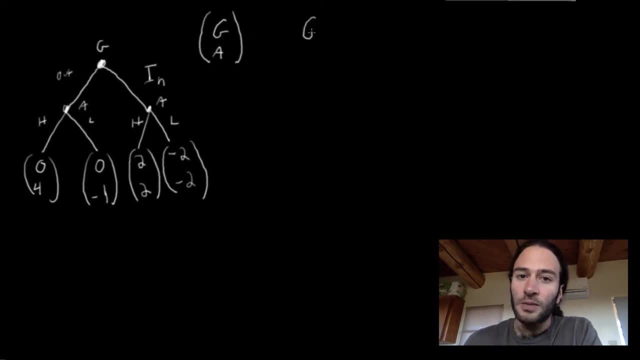 strategy profile now here. This strategy profile is going to be that Google plays out and Apple- remember now Apple strategy. I'll put GS for strategies. Apple plays. if out, then choose the high price. If Google plays in, then choose the low price And what we want to. 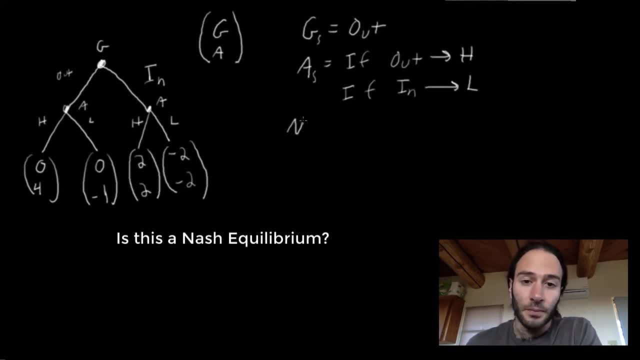 see is: is this a Nash equilibrium Any Now? remember the definition of a Nash equilibrium before. No player has an incentive to unilaterally change its strategy. So to see if this is a Nash equilibrium, we just need to check to see if any player has an incentive to changing its strategy, leaving 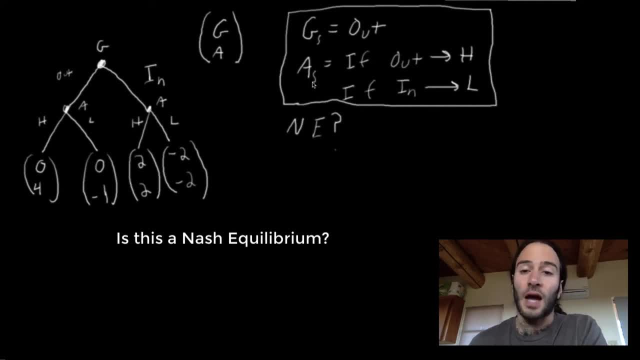 the other strategies of the other players constant. So let's first look at Google. If Google, if Google's playing out and Apple plays high price, if Google plays out, Google gets zero. Now does Google have an incentive under this strategy profile for Apple to change? 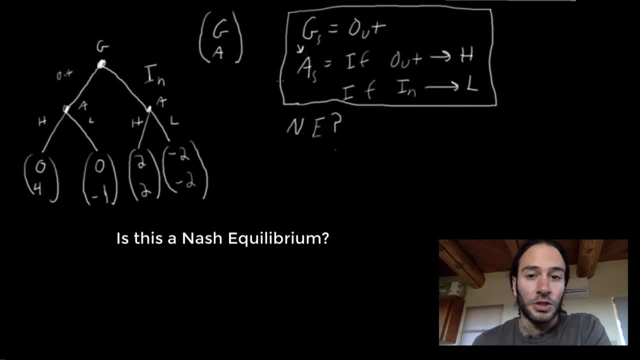 its strategy to in. Well, if it changes its strategy to in, Apple will have a low price. So Google would get negative two. Because negative two is worse than zero, Google does not have an incentive to change its strategy. You should keep the other play Entering. yes, pleased news. Remember when looking. 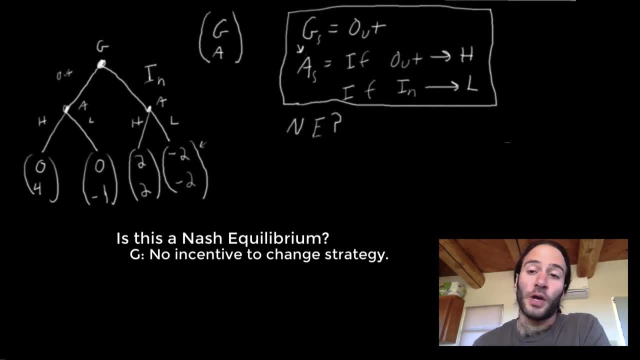 at incentives to change strategy. you always keep the other player's strategy constant. So how about for Apple? If Google plays out, Apple can change its strategy. Now look, no matter what Apple changes its strategy to, here for the if in part of the strategy, its 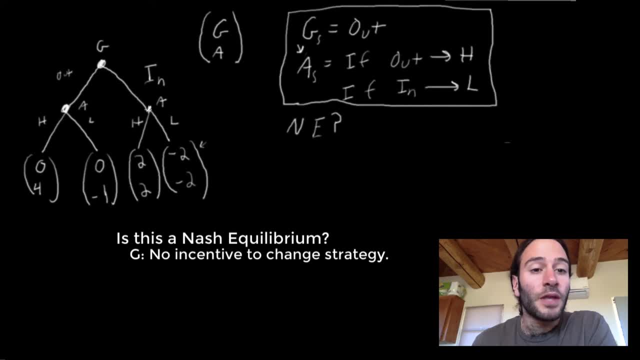 payoffs won't change Because if Google is playing out, we will never reach this decision. node strategy is fixed to playing out. Apple will never have to make a decision, as if Google plays in. So changing Apple's strategy condition on Google playing in.